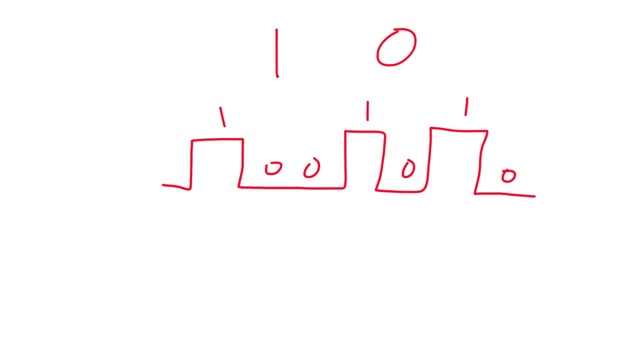 So how do you store or represent, say, the number 25 as a pure binary integer? First let's look at the number weighting line that we are familiar with and we've grown up with since primary school. Our number system is called DINERY. It's a base 10 number system. 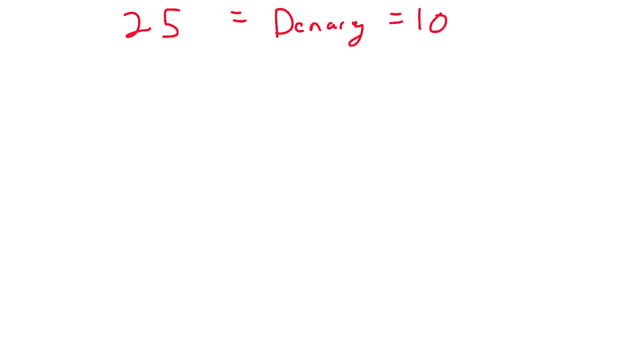 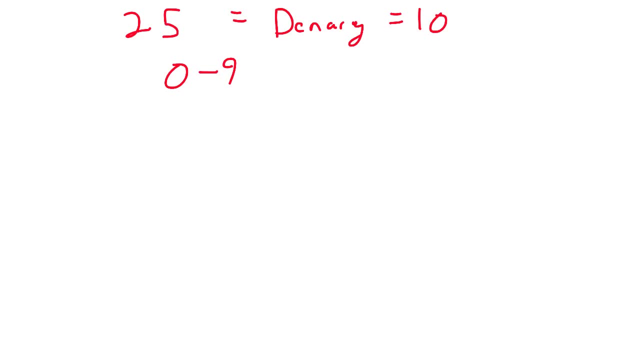 other numbers in our system are made up for combining these numbers together. Because of this, the DINERY number weighting line multiplies by 10 every time we move to the left. Our first column has a weighting of 1.. Our next column has a weighting of 10s. 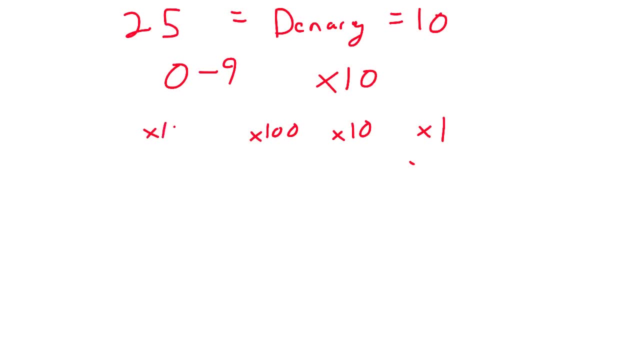 Then a 100s, Then a 1000s, And so on and so forth. The number 357 is stored as 3 lots of 100 plus 10, lots of 5 plus 7, lots of 1s, With a binary or base 2 number system, the 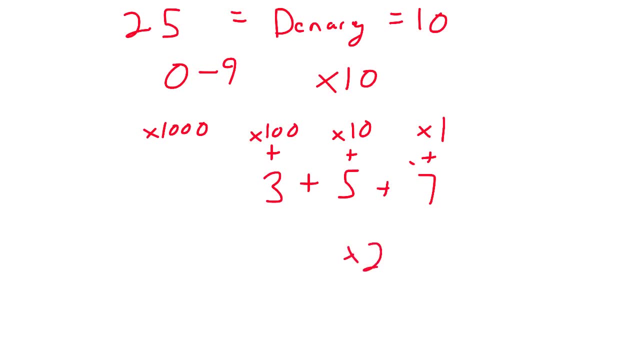 number weighting line, therefore, is a binary number system. The number weighting line, therefore, is a binary number system. The number weighting line, therefore, is a binary number system. TheQu advertises that an observant must multiply 100 times its number up by 2. 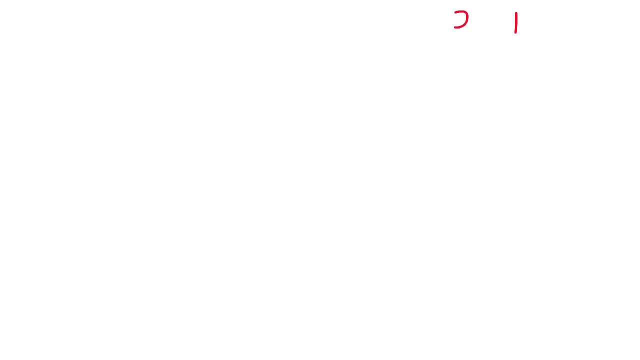 every time it moves to the left. TheQu advertises that an observant must multiply 100 times its number up by 2 every time it moves to the left. The invov 카메라, which asks questions such as how welands the degree of Manufactured. 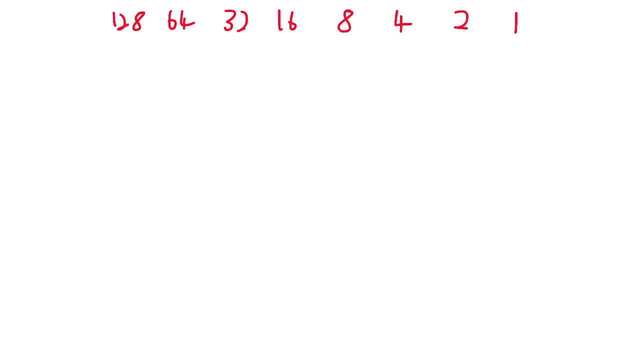 кажется. totality was finally answered with this…. Every time we go up, we're doubling thanks to a base 2 number system. Next, we want to be sure that we're getting a good sort of passing record When we get. So let's go back to our question and let's see how we fit the number 25 into binary. 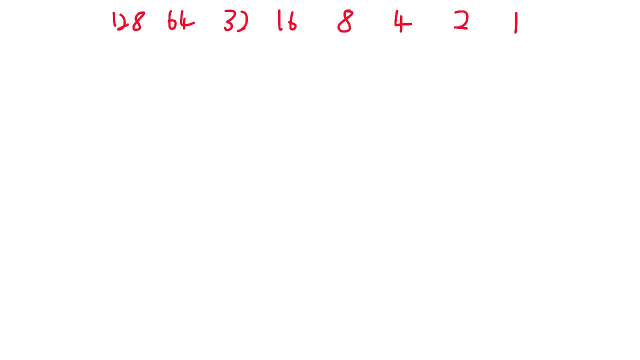 The first thing we have to do with this weighting line here is say: how many 128s can you fit into 25?? We're starting on the left. The answer, of course, is that no 128s will fit into 25.. So we write 0 under this column. 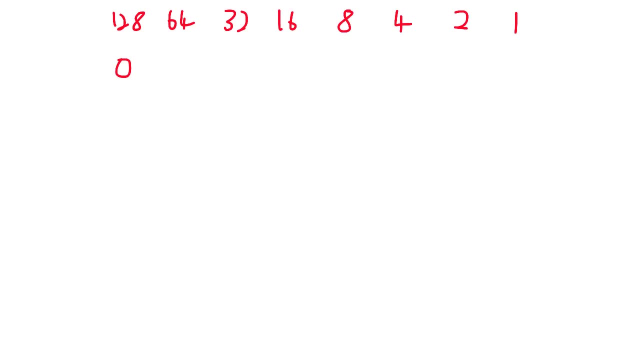 Next we look at how many 64s you can fit into 25.. Again, the answer is 0.. How many 32s can you fit into 25?? Again, it is 0.. Now we get to the 16 weighted column. 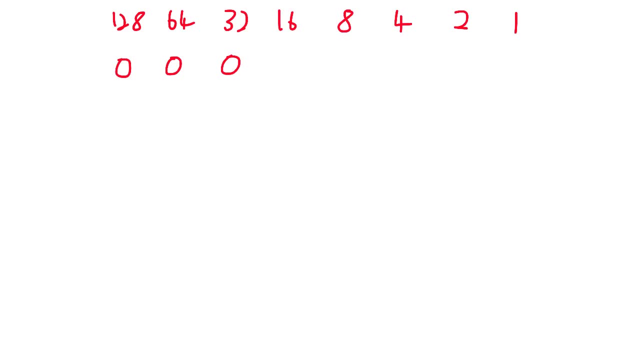 How many 16s can we fit into 25?? The answer is 1. so we write 1 under that column and we have 9 now left over. We now move to the next column. We have 9 left over. How many 8s can we fit into 9?? 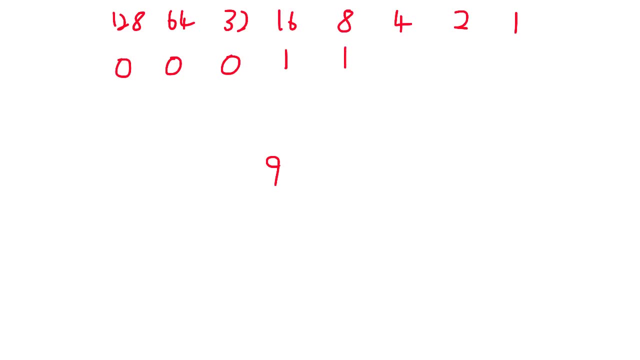 The answer is 1, so we write 1 under the column and we have 1 left over. We now go to the 4s column. How many 4s can we fit into 1? 0. We still have 1 left over. 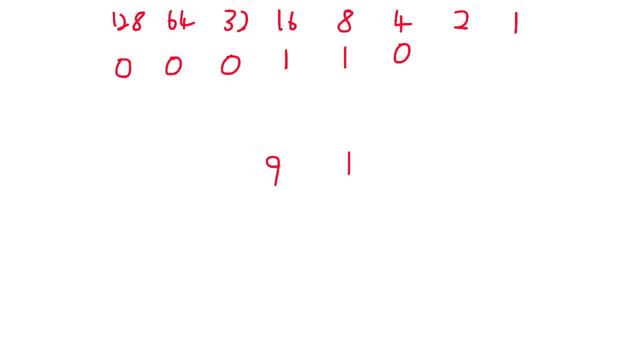 How many 2s can you fit into 1?? It's 0 with 1 left over. And finally, how many 1s can we fit into 1?? The answer, of course, is 1 with nothing left over. So the deanery number of 25 in binary is 0.. 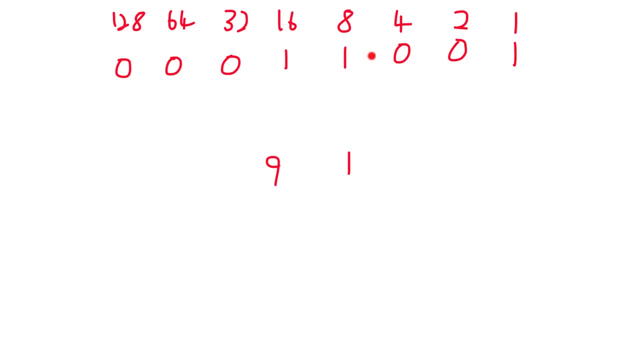 That's it. The answer is 1 1 0 0, 1.. We can prove this by adding up the weight of the columns that have 1s in. We have a 16 column plus an 8 column plus a 1 column, and 16 plus 8 plus 1 equals 25.. 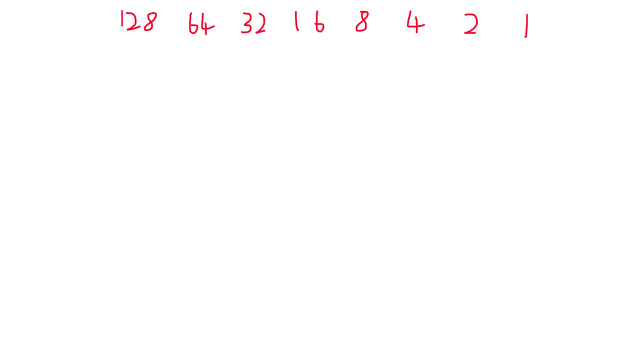 Your turn to have a go. Pause the video and try to do the reverse: Translate the pure binary integer 0, 1 0, 0 0, 1, 1, 1 into deanery and see what you come up with. The first thing you should have done is taken the binary number and placed it underneath the base 2 binary weighting line. 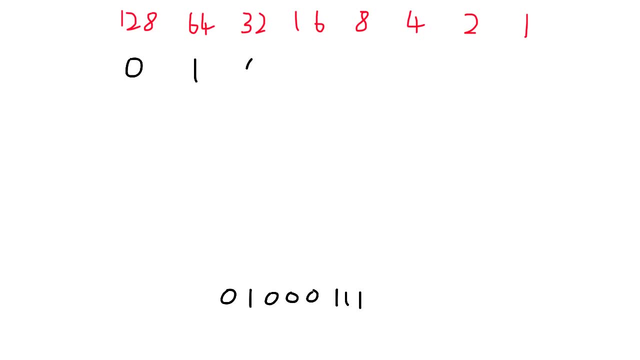 So you go 1 0 0, 1 0. 1 0, 1 1 into the first binary integer. That's it. Ok, now for the test. This is for the played out third number. This is the number that was taken later in the trilogy.